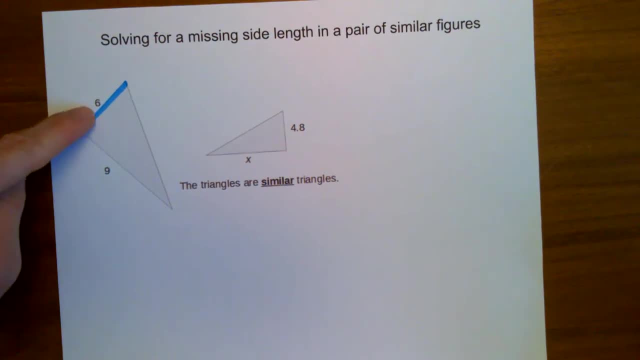 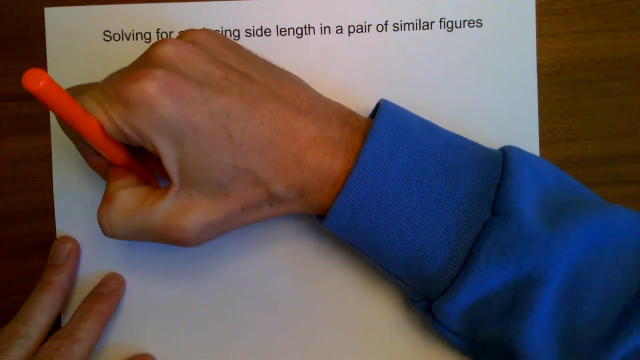 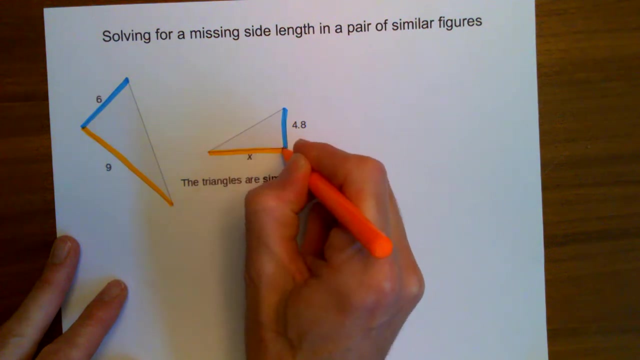 one is the shortest side, So that needs to match up with the shortest side of this one, And then it looks like this side length is a nine over on this larger triangle. That would be the medium size length of that triangle. So the medium size length, the medium side length of this one, is: 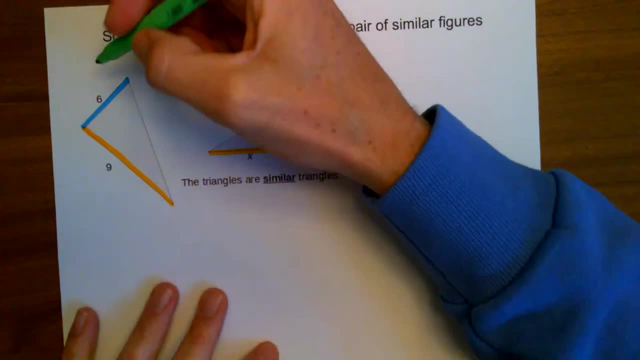 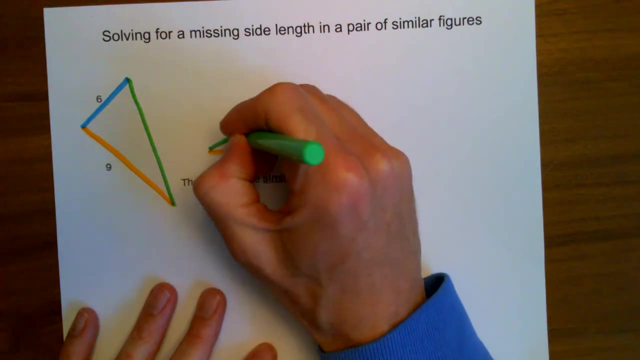 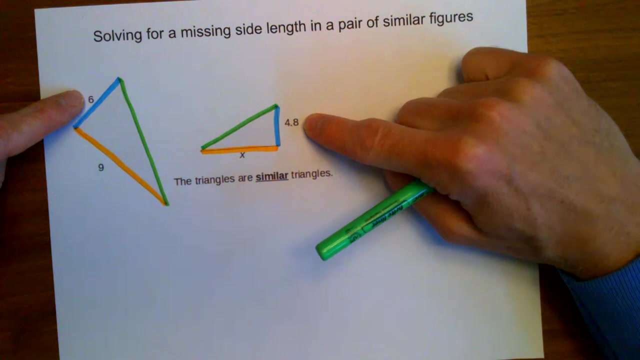 going to be orange over here And that leaves the largest side, the longest side. I'll color in green And that's going to match up with the longest side of this triangle in green. So now I know the six and the 4.8 go together And the nine and the unknown go together. So going back to 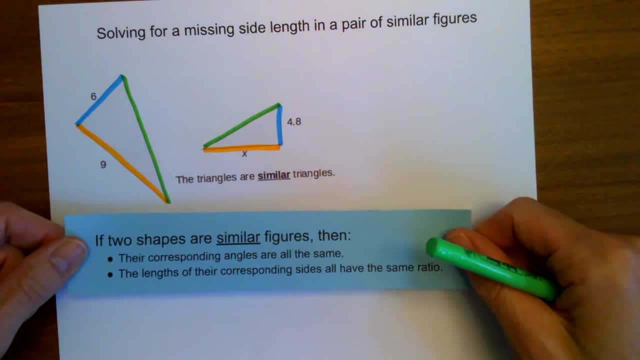 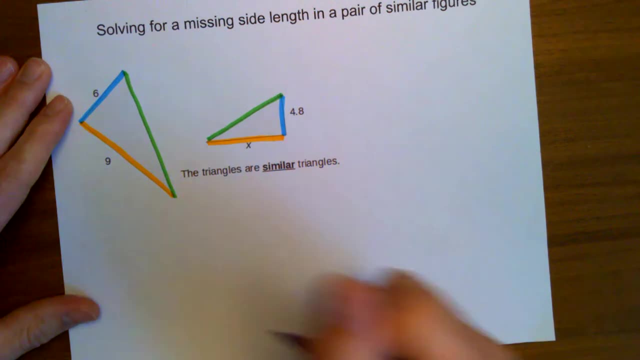 this one. the ratio of the corresponding sides must be the same. They have the same ratio. So here's how I'm going to write my ratio for this one. There are a couple ways you can do it, But I'm going to write the ratios this way. I'm going to write my ratio as the let's go. 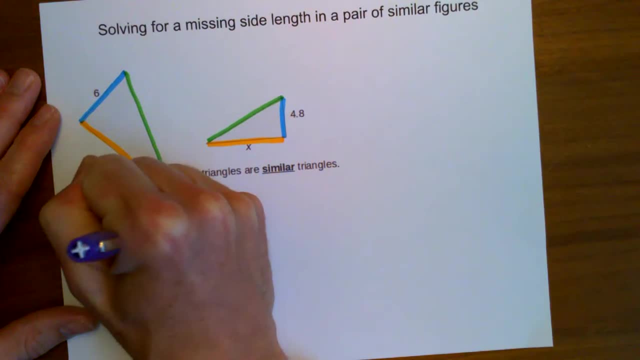 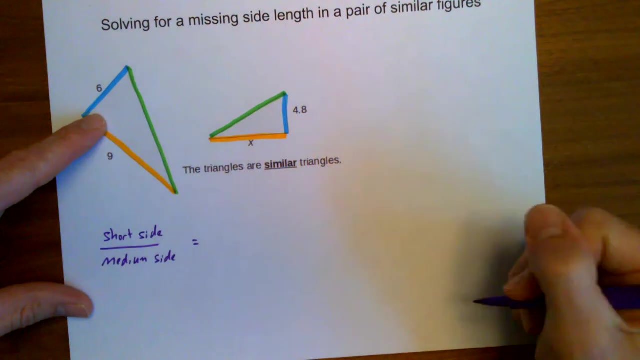 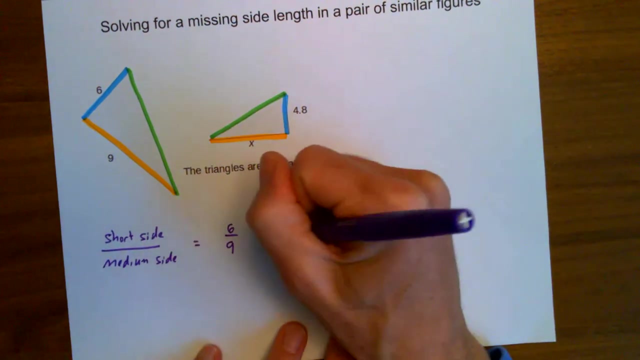 the ratio of the short side to the medium side. That's my ratio that I'm going to write for each of these triangles. And so for the larger triangle, that ratio is six to nine, And for the smaller triangle that ratio is short side to medium side, That is. 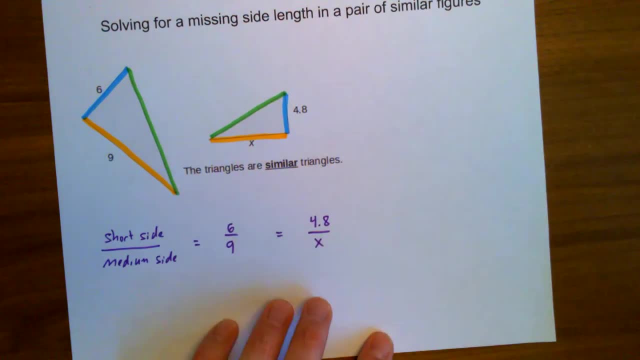 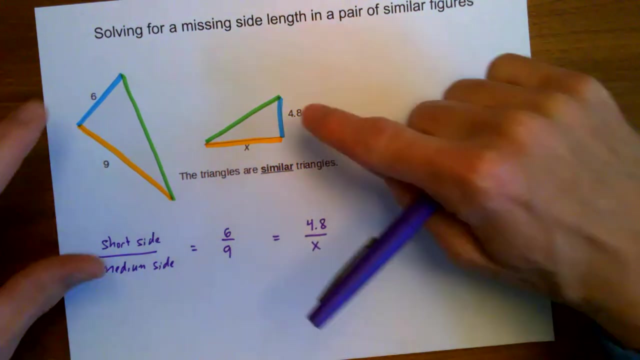 4.8.. To unknown. So these two ratios are the same. I need to figure out what this one is, And the method I'm going to use is I'm going to figure out what is the scale factor that takes me from this one to this one. I know that this triangle is smaller, So this blue side shrunk from six to. 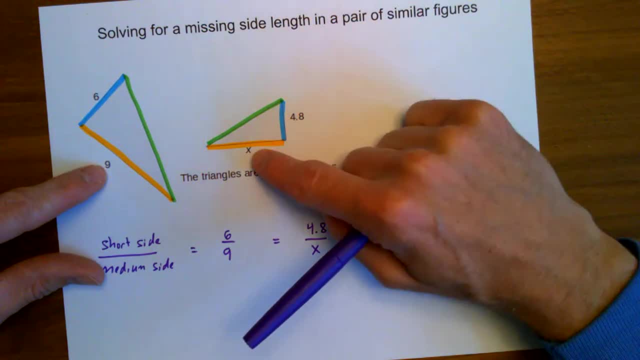 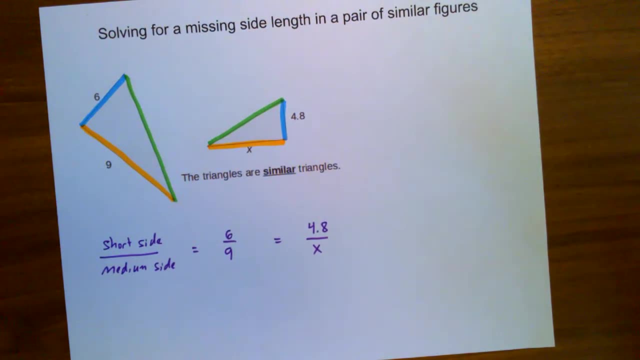 4.8.. So the nine must shrink from nine down to something else. So it's going to be less than nine, But it's got to be more than nine. So it's got to be less than nine, But it's got to be more than 4.8.. So I'm just kind of thinking through this one a little bit. 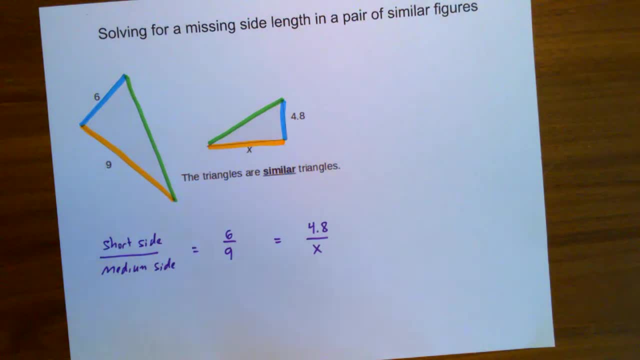 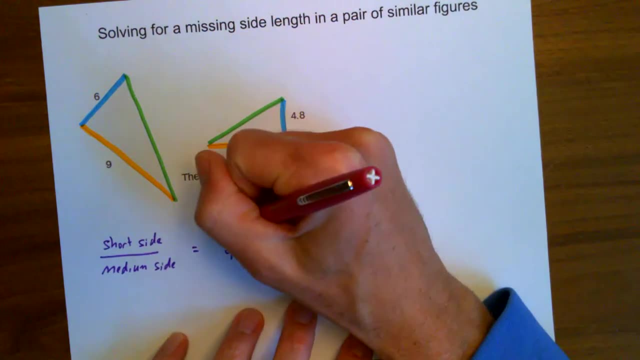 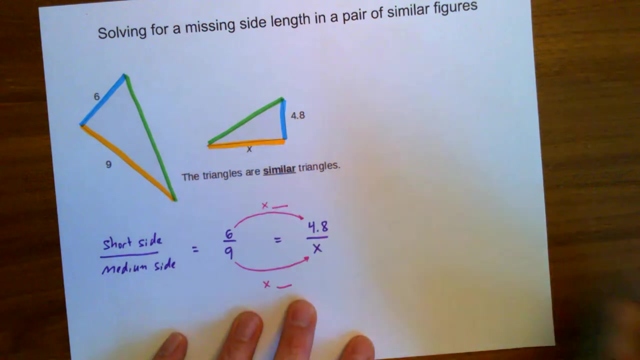 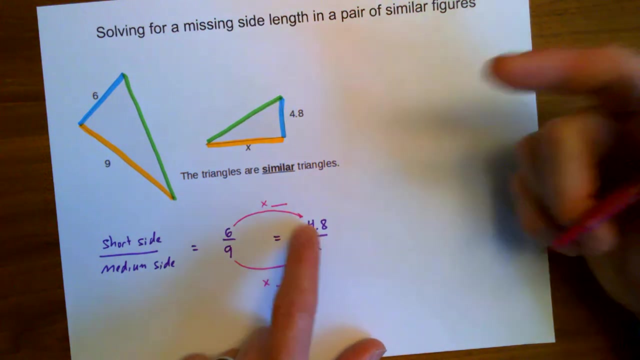 And the way I'll do this is: let's find a scale factor. In other words, what number am I multiplying these sides by to get these sides? So what am I multiplying by to get the new side lengths? So, six times something equals 4.8.. Well, what is that something? Let's work back. 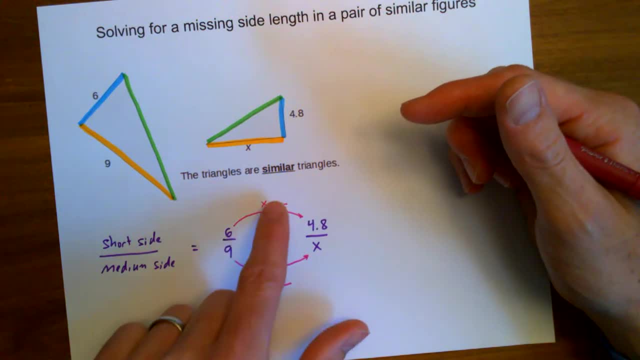 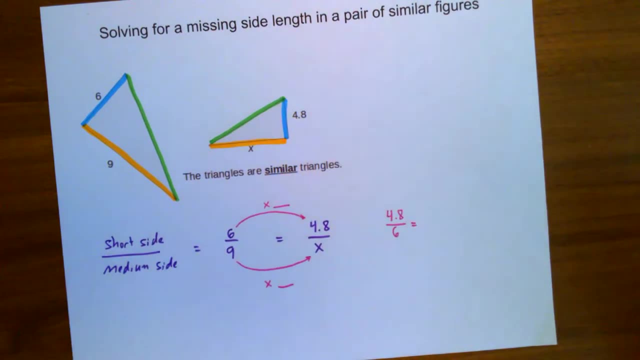 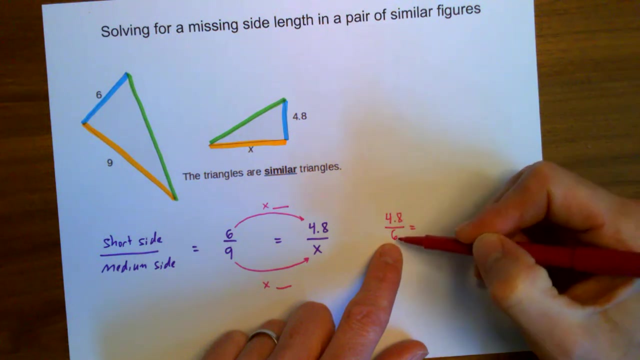 Where's the opposite of multiplying is dividing Instead of six times something is 4.8, I can do: 4.8 divided by six equals that something, So I can use my calculator at this point. By the way, I also, just based on the numbers here, I know that six times eight is 48. So six times 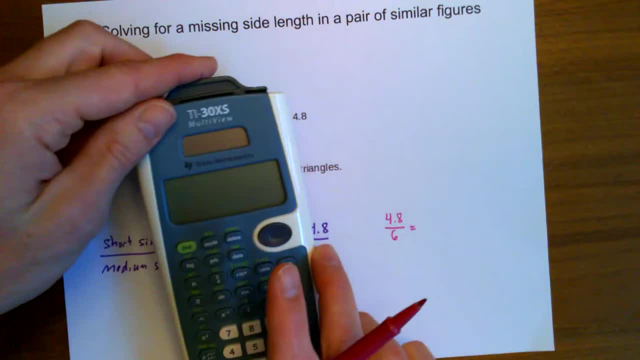 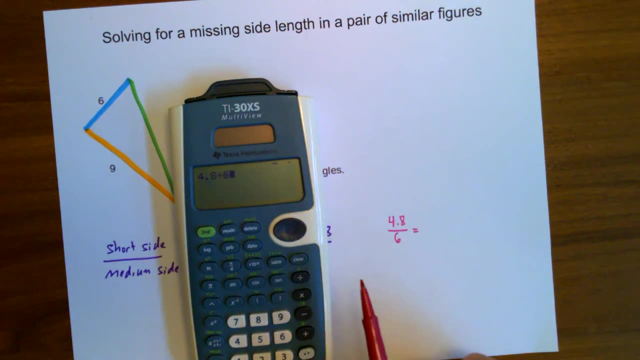 .8 or eight-tenths should give you 4.8.. But just to confirm, I'm going to use my calculator at this point. Let's check: 4.8 divided by oops, not multiply. divided by 6, equals 0.8, 8 tenths. 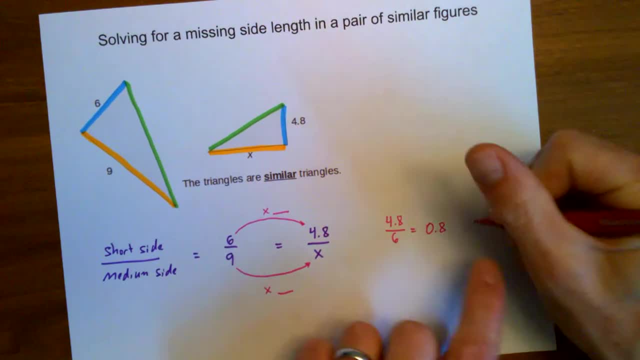 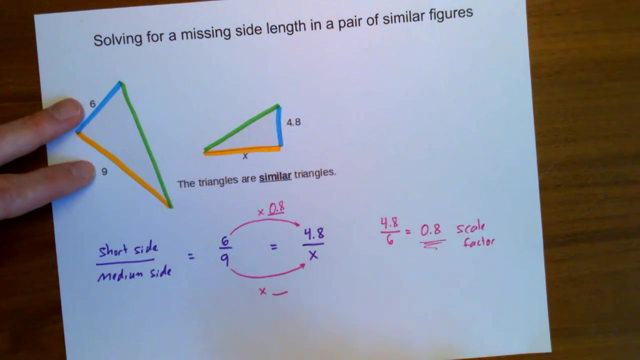 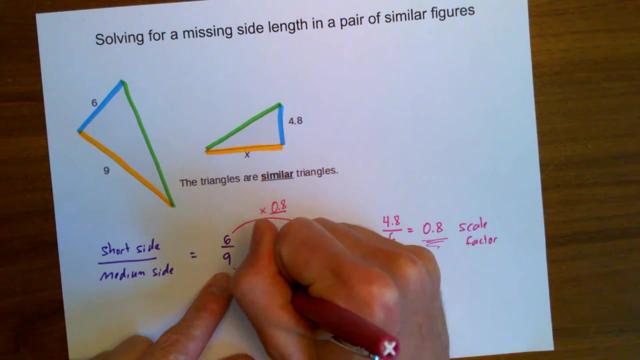 So I know now that my scale factor- sorry about the scratchy markers here- the scale factor- must be 0.8.. So we're multiplying these side lengths by 0.8 to get the smaller new side lengths. So let's multiply this one by 0.82.. 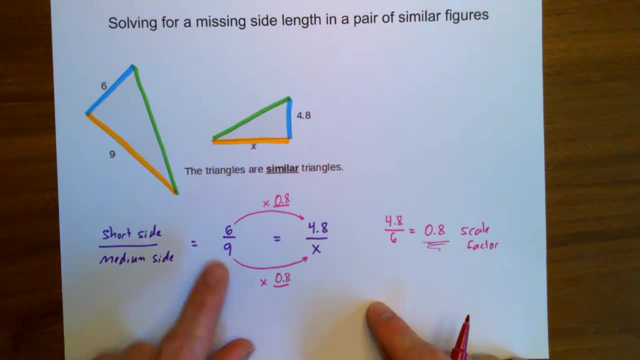 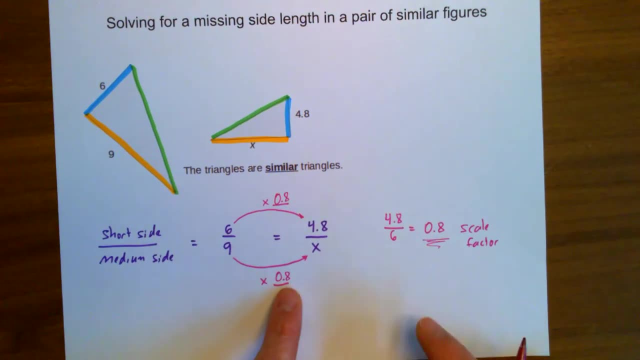 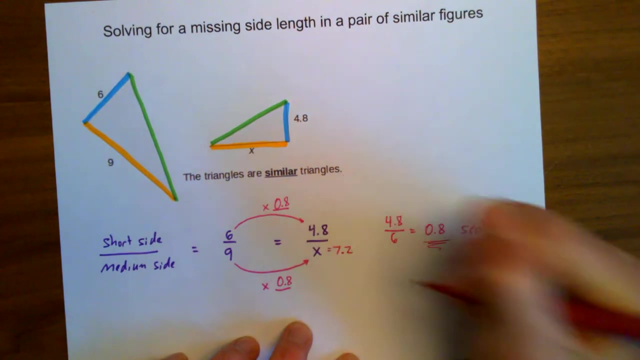 9 times 0.8 should tell me the new side length. And can we do this without a calculator? You can use a calculator if you want, But I know that 9 times 8 is 72.. So 9 times 0.8 should be 72.. 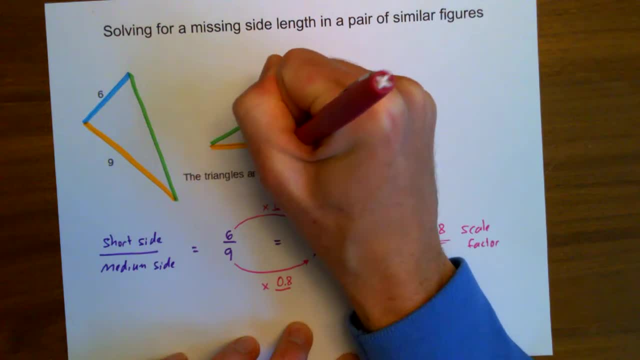 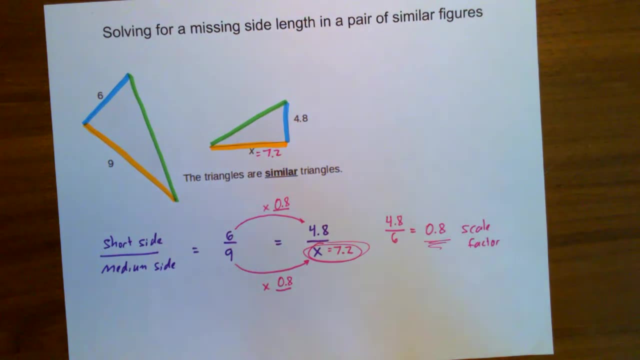 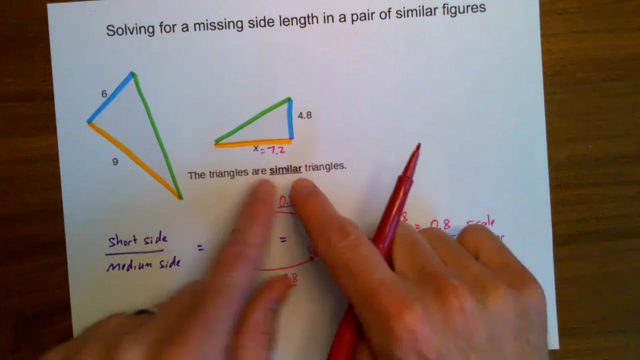 So this new side length over here has shrunk from 9 down to 7.2.. 7.2 is my answer. So I have solved for this missing side length, knowing that the ratios of these sides needs to remain the same if these are a pair of similar triangles. 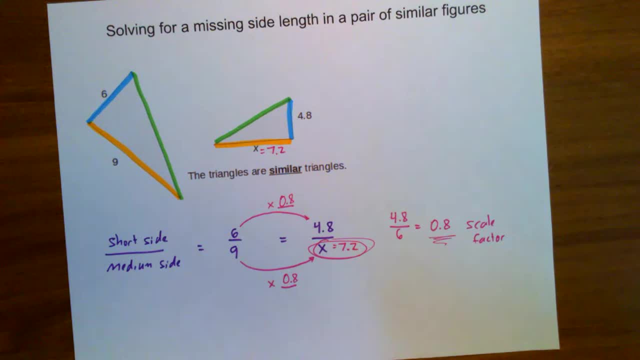 The problem says they are, so I can use that ratio to solve. So hopefully that helps when you are dealing with similar figures.